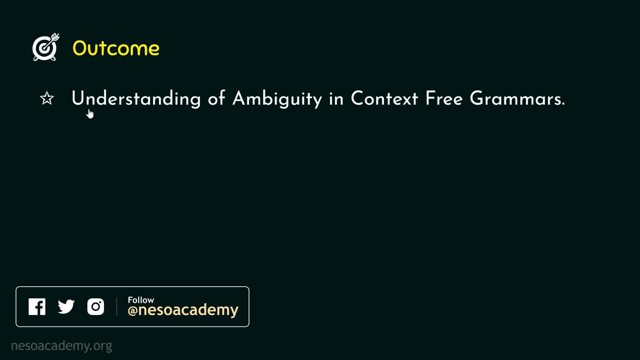 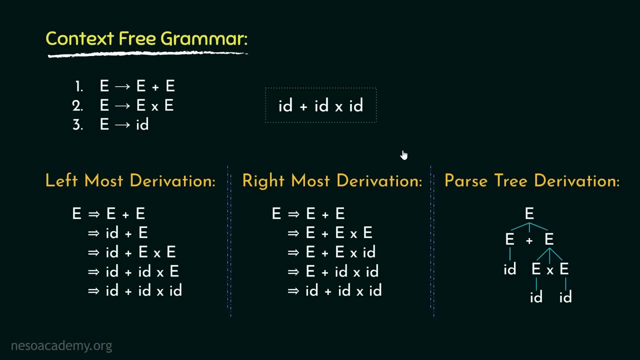 Coming to the outcome of this session. today we will acquire the understanding of ambiguity in context-free grammars with the help of an illustration. Now, if you all remember, in the previous session, with the help of this grammar, we wanted to derive this string of terminals. We also observed that using the leftmost 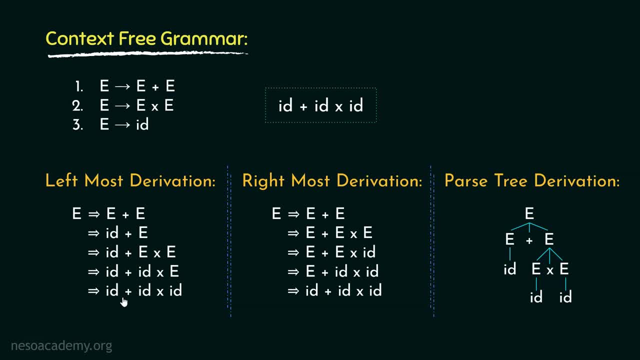 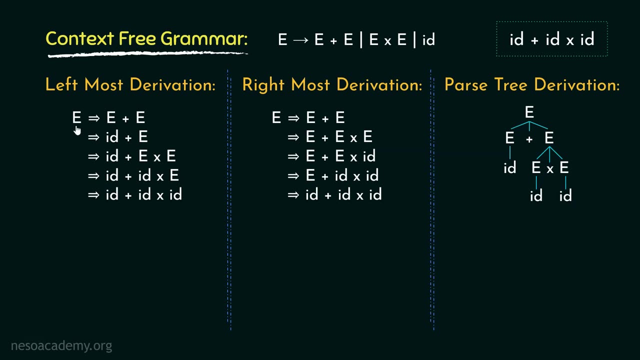 rightmost and parseTree derivation, we finally achieved our intended string. Let's now observe if there is any other way to derive the same string using these procedures. Let's begin with the leftmost derivation method. Now, the last time. from the start symbol e we derived e plus e using the rule e can be. 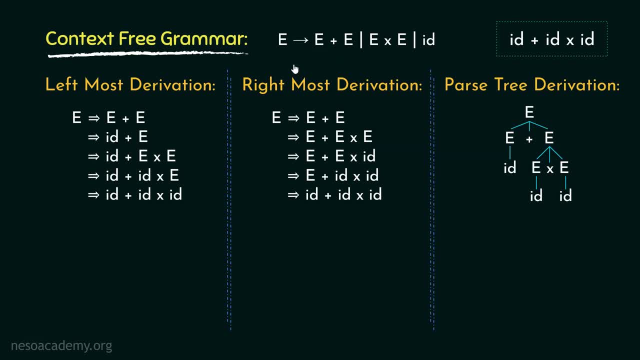 rewritten as e plus e. This time let's use the next rule: ie e can be rewritten as e into e, So from e we derive the sentential form e into e. Now, this is leftmost derivation procedure, so we will be concerned about the leftmost. 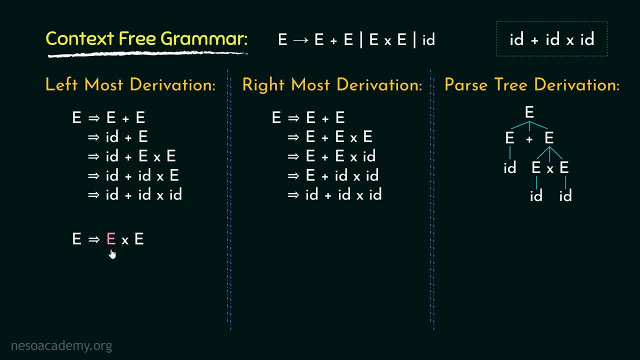 variable, which in this case is this one. Now observe the string. We have acquired the multiplication operator and now we need the addition operator, right? So this time we will use this production. ie. e can be rewritten as e plus e. So, expanding the leftmost e, our derivation becomes e plus e into e. 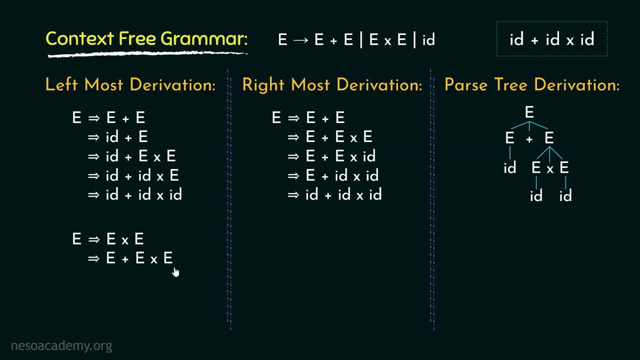 and now we have achieved the format From all these. this is the leftmost non-terminal and we will simply derive id from this, because the format is already achieved. Now, from these two, this is the leftmost one, so we will derive id again. 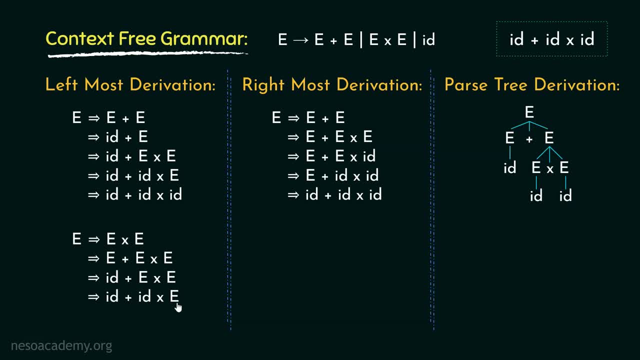 Now we are left with only one e. Let's expand this one. So we now have derived the string id plus id into id. Well, this is the intended string. So observe: although we started off with different production rules, by the end we ended up. 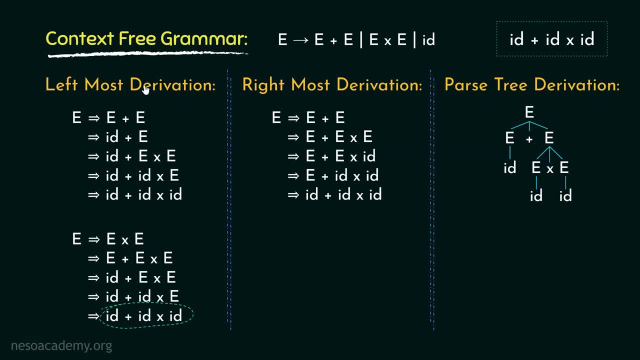 achieving the same result. So there are more than one leftmost derivations for this particular string. Let's now observe whether that's also the case for rightmost derivation. So here also we will start off with the second rule. so e derives e into e. 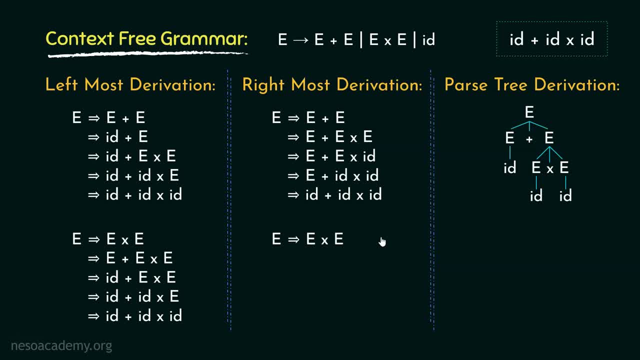 Now remember, this one is the rightmost derivation. And from these two, this is the rightmost one. If we notice the string after the multiplication operator, we have id. So expanding this e, we will derive the sentential form e into id. 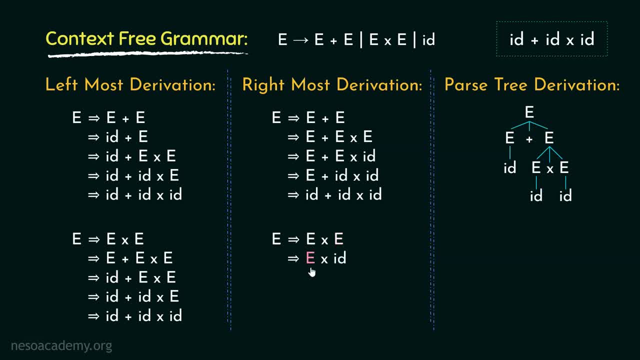 Now there's only one non-terminal, So let's expand that. Notice that we have covered the last portion and we are yet to derive this portion. So from this e, Using the first rule, we will derive the sentential form e plus e into id. 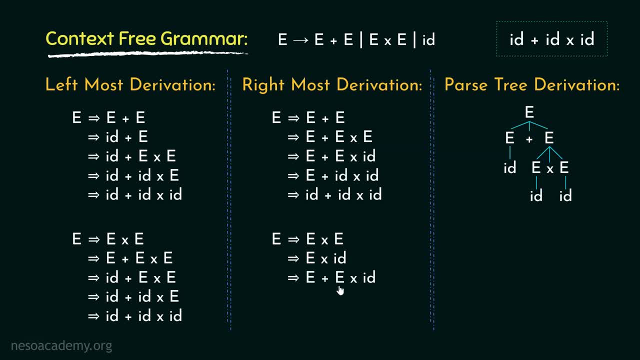 Now there are two e's, and among them this is the rightmost one. Since we have achieved the format already using the third rule, that is, e can be rewritten as id. we will derive the sentential form e plus id into id. 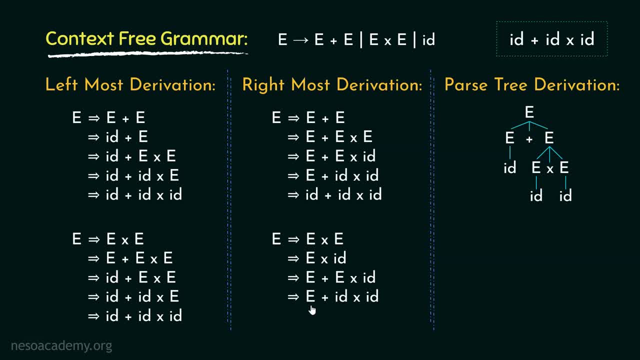 So we are almost there. Now all we have to do is expand the only one. So finally, we will derive id plus id into id, And this is the intended string. So, similar to the leftmost derivation, there are more than one rightmost derivations for. 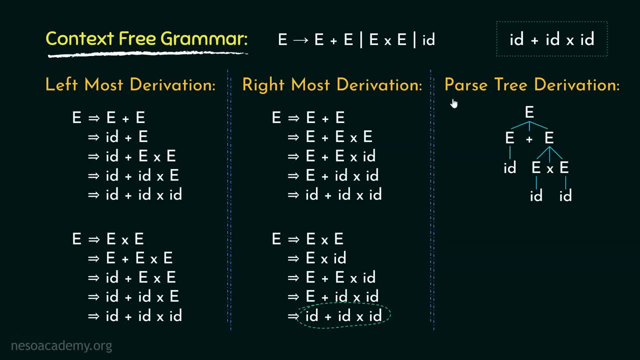 the same string. Let's see if that's also the case for the parse tree derivation. So we will start off with the start symbol e. Now, unlike the last one, This time Let's derive e into e. From this, Now, from this e, we will derive e plus e. 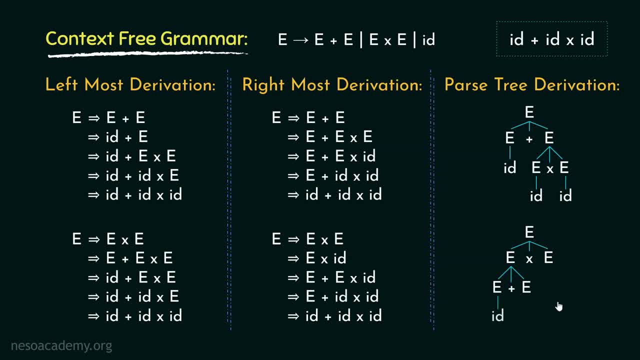 And finally, from all these e's we will derive id's. So if we traverse the tree top to bottom and left to right, the yield would be id plus id into id. So yes, there are more than one parse tree for the same string. 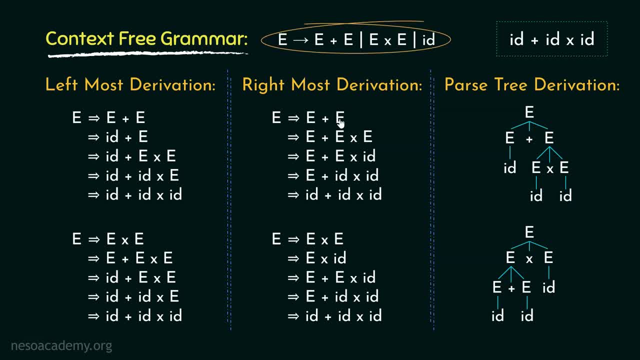 Now remember this: For any grammar, If we obtain either more than one leftmost derivations or more than one rightmost derivations or more than one parse tree, then the grammar is clearly ambiguous. If it had been unambiguous, the derivations should have been unique and one and only.